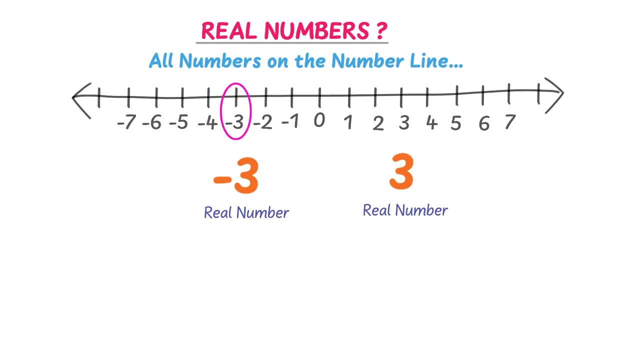 be spotted or plotted on a number line. It is a negative integer. Now, what about 2.5 and minus 2.5?? Well, they both are real numbers because we can spot them on a number line. Also, what about 25 by 100 or 0.25?? 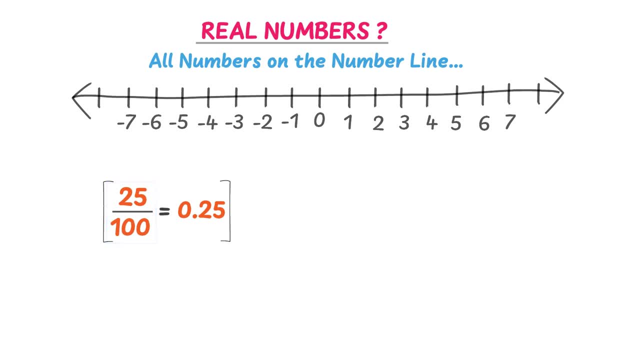 Can you guess it? Well, 25 by 100 is a p by q form, where q isn't equal to 0, and 0.25 is an example of terminating decimal. Now, what is terminating decimal? A decimal which has finite number of digits and its decimal part. 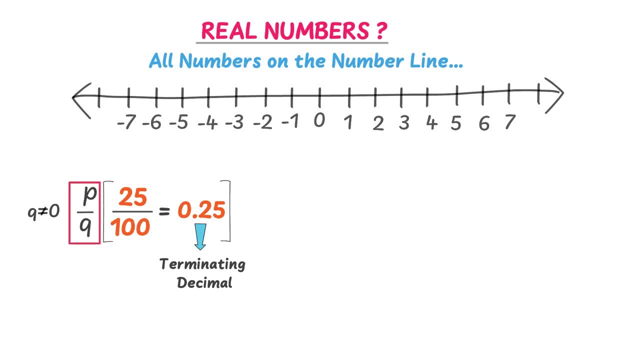 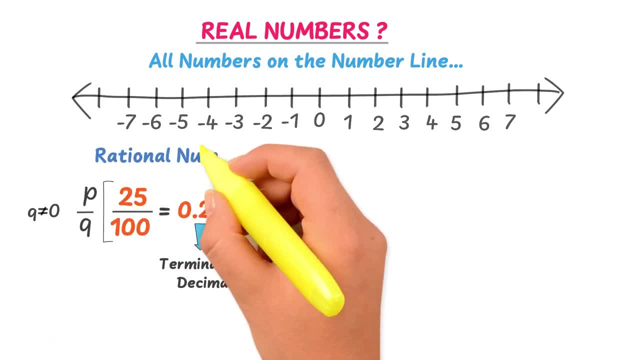 So 25 by 100 is a number which we can write and p by q form. It has terminating decimal, Thus it is a rational number. We can spot our plot 0.25 on a number line. So 25 by 100 is a real number. 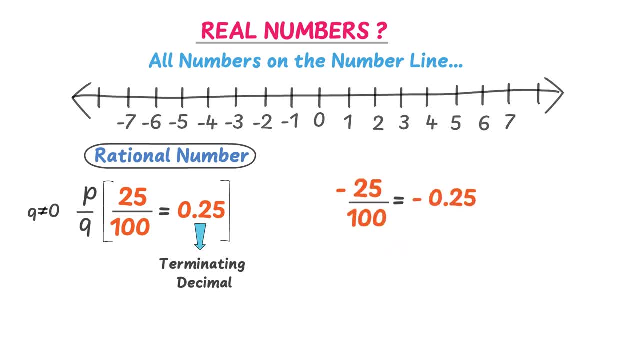 Similarly, minus 25 by 100 or minus 0.25 is also a real number because we can spot our plot it on a number line. Now let me ask you what you have learned from this example. Well, we learned that all rational numbers are real numbers because we can spot our plot. 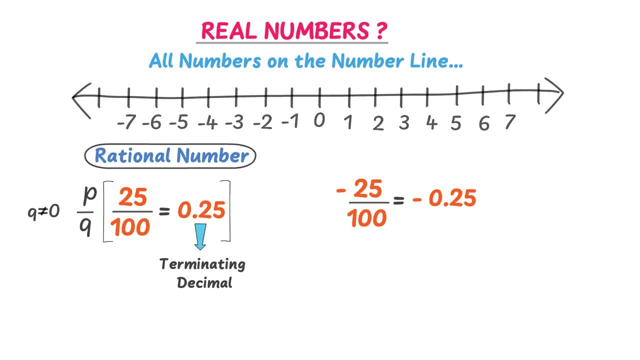 them on a number line. Thus, all rational numbers like 1 upon 3,, 2 upon 6,, 200 upon 3 are real numbers. Finally, what about root 2? Is it a real number or not? Well, root 2 is equal to 1.41421.. Well, root 2 is equal to 1.41421.. Well, root 2 is equal to 1.41421.. So it is a rational number, with care to preach論 4.. Let us put rows of 1,, 3, and so on.